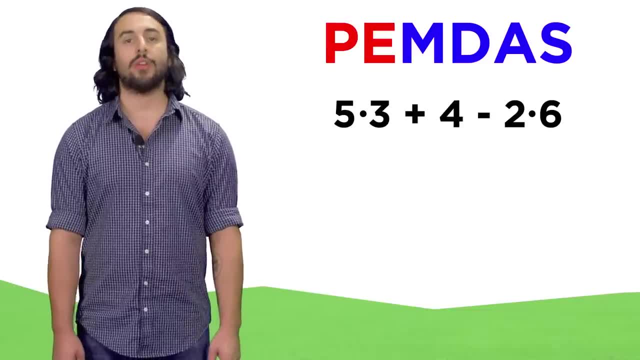 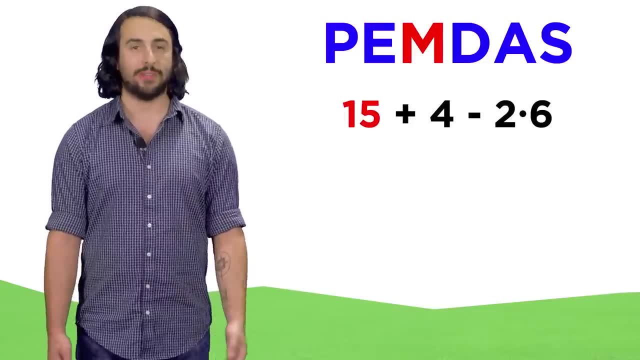 Let's apply this method to our previous example. There are no parenthetical terms or exponents, so let's jump straight to the multiplication. Five times three is fifteen, That's fifteen, And two times six is twelve. We must do this before doing any addition. 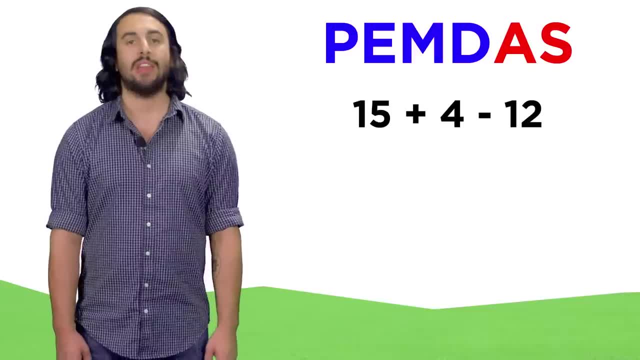 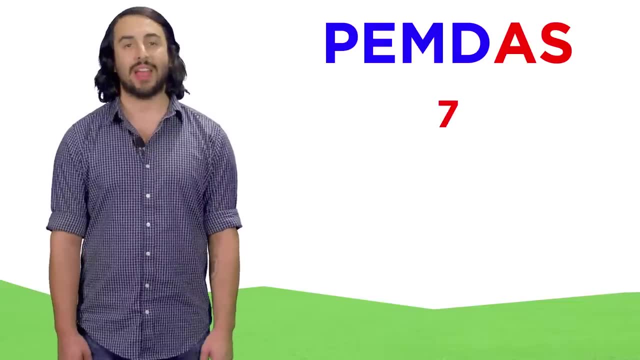 Now this reads: fifteen plus four minus twelve. Now it's all addition and subtraction. so we just go left to right: Fifteen plus four is nineteen minus twelve is seven and according to PEMDAS, this is the only correct answer. 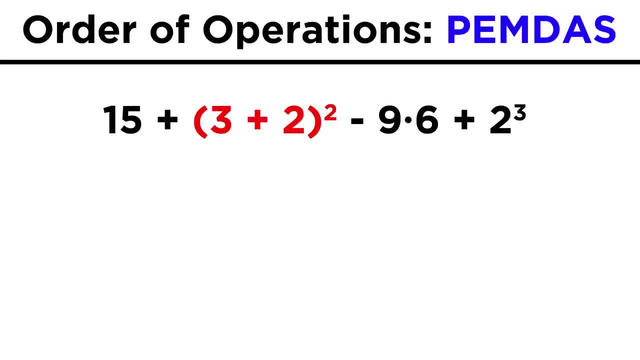 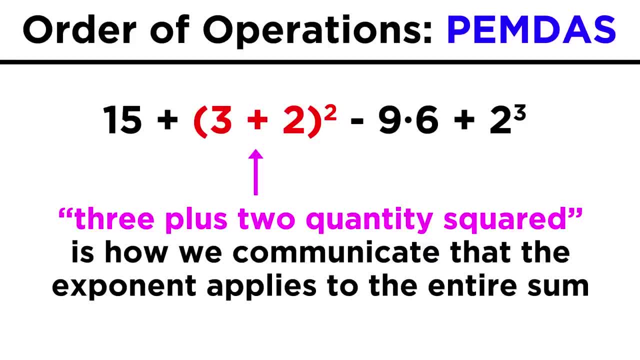 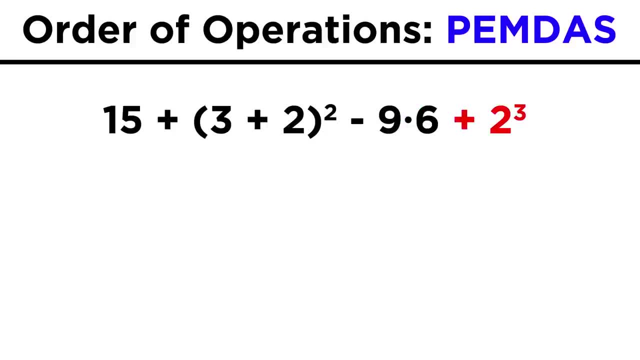 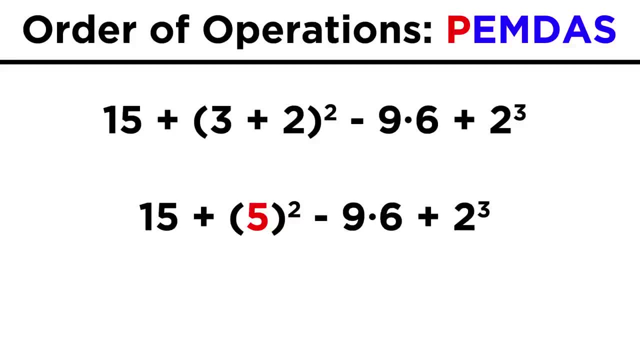 First we do the parenthetical term: three plus two is five. Then we do any exponents: Five squared is twenty-five and two cubed is eight. Now we have to do the multiplication before we do any addition. so nine times six is five. 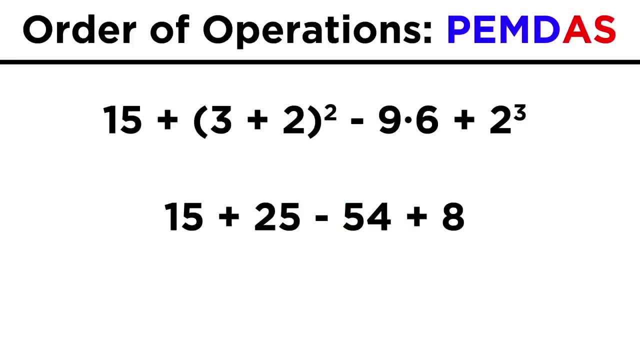 Now we can just add and subtract across. Fifteen plus twenty-five minus fifty-four plus eight equals negative six. This is the only correct evaluation of this expression when we follow the order of operations. If you want to make sure you can do this on your own, let's check comprehension. 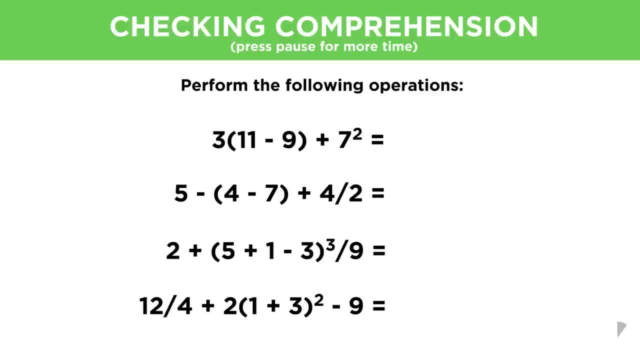 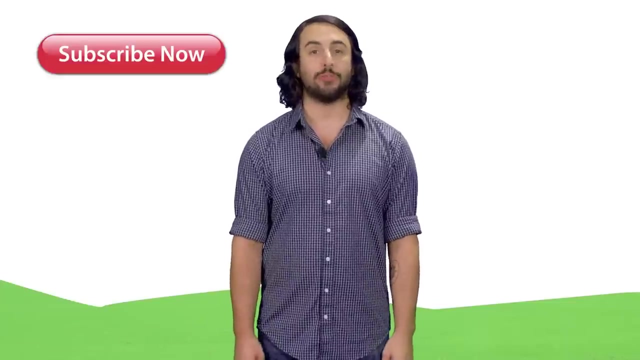 If you want to make sure you can do this on your own, let's check comprehension. If you want to make sure you can do this on your own, let's check comprehension. Thanks for watching, guys. Subscribe to my channel for more tutorials. 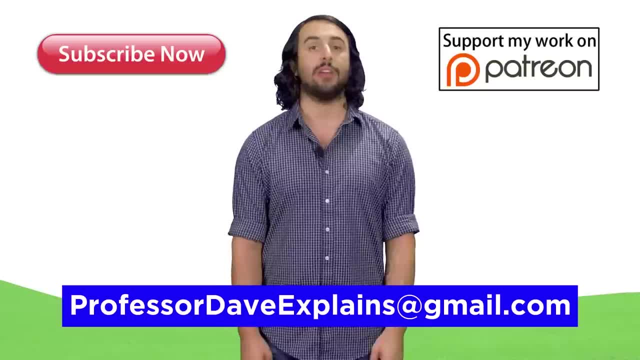 Support me on Patreon so I can keep making content and, as always, feel free to email me professordaveexplains at gmail dot com.